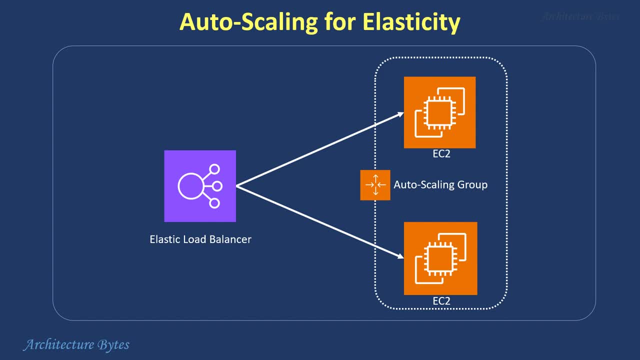 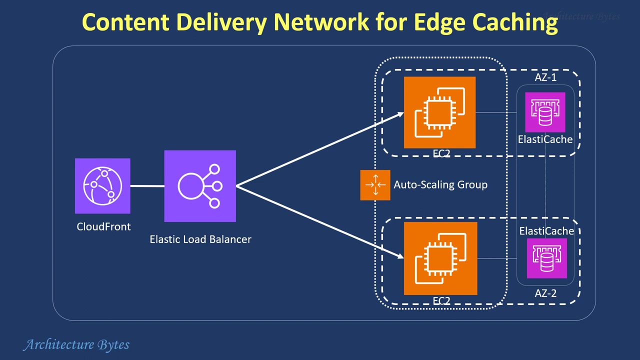 This ensures that the application can handle varying load efficiently. Use multiple availability zones, with the auto-scaling group spread across them to ensure redundancy and high availability. Use Amazon Elastic Cache to cache frequently accessed data, thereby improving data read performance. Utilize Amazon CloudFront, a content delivery network, to cache and deliver static and dynamic content from edge locations, thus reducing content delivery latency and improving user experience. 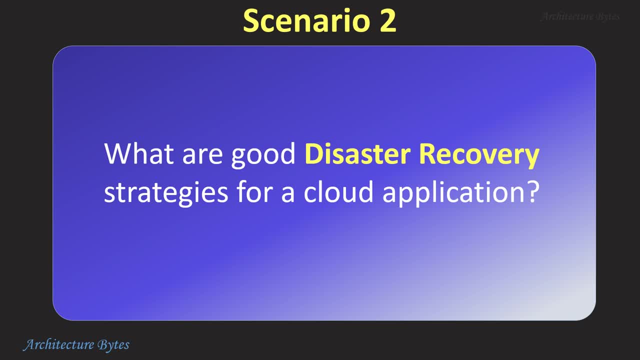 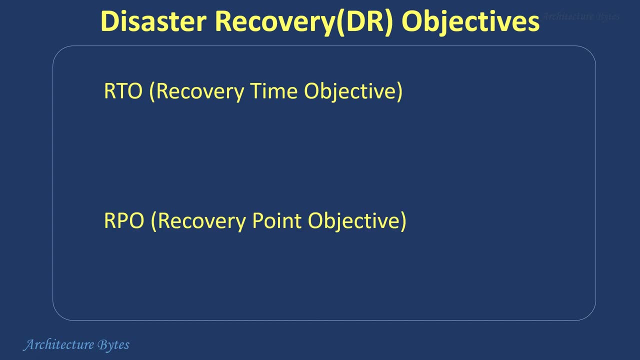 What are good disaster recovery strategies for a cloud application? Our disaster recovery strategy should be based on RTO and RPO. Let's understand these terms first. RTO or Recovery Time Objective. RTO is duration within which a business process must be restored. 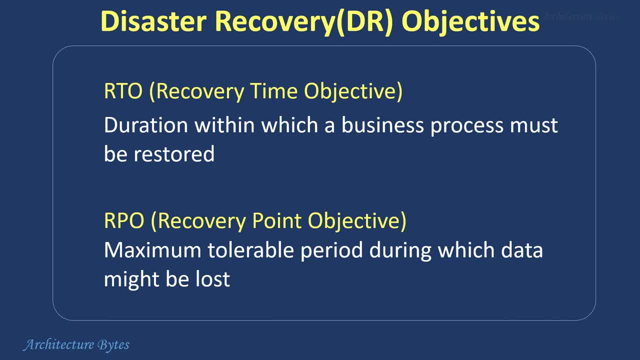 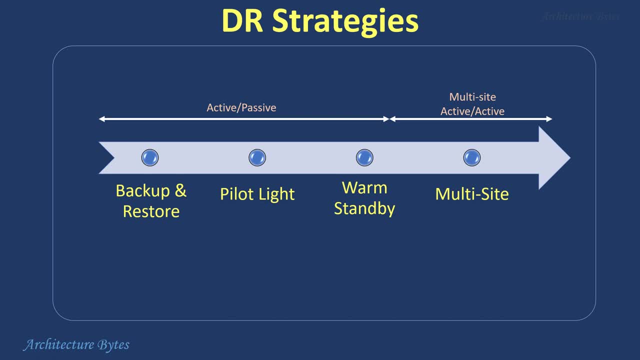 RPO or Recovery Point Objective. RTO is maximum tolerable period during which data might be lost. Keeping these in mind, common DR strategies are: Backup and Restore, Pilot, Light, Warm, Standby, Multi-Site, Each varying in RTO-RPO time and costs involved. 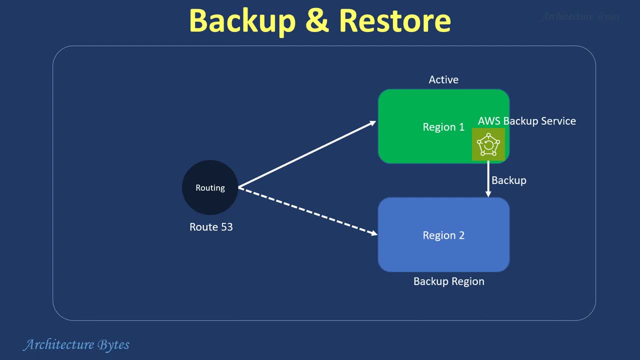 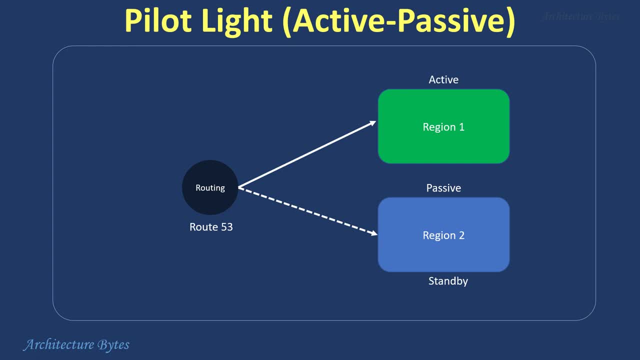 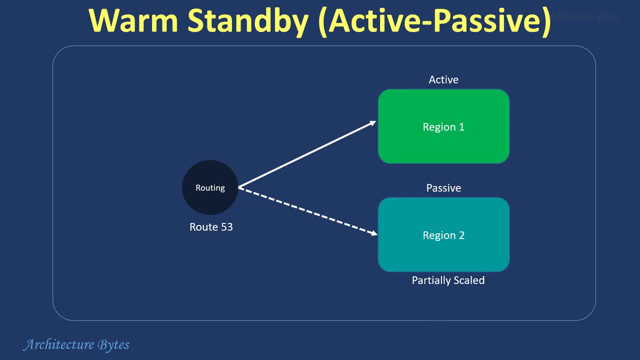 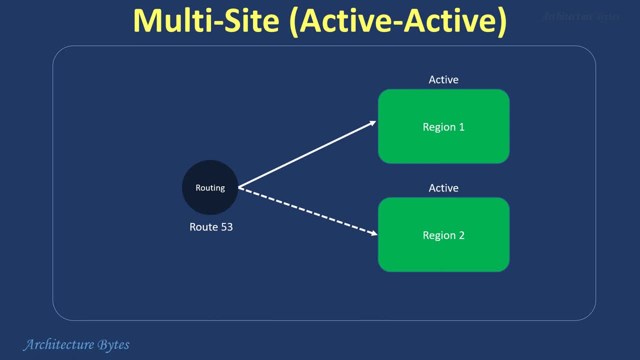 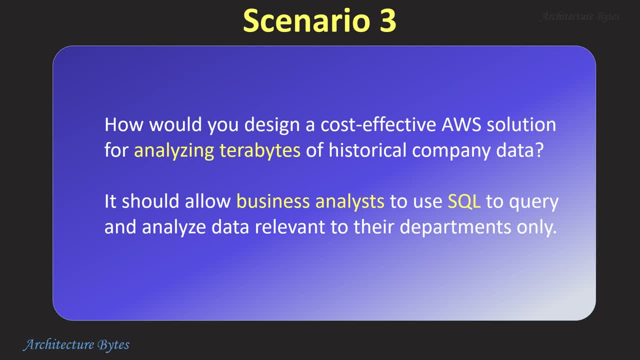 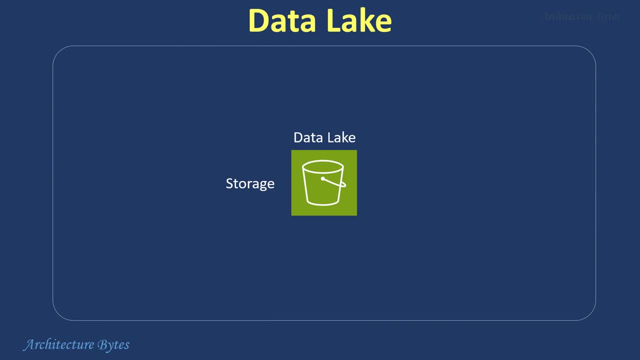 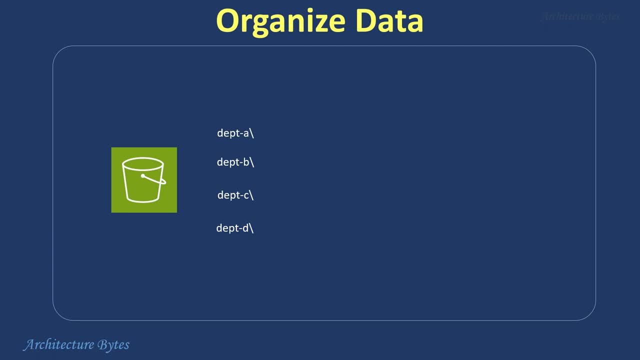 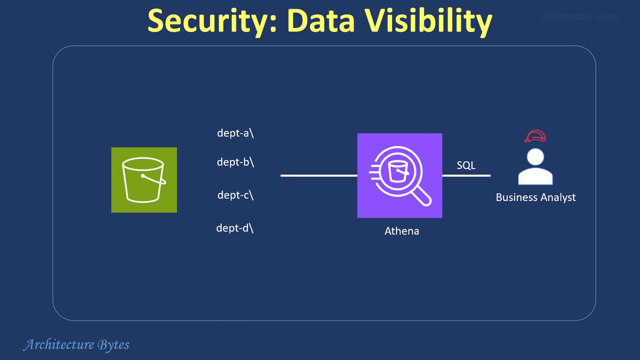 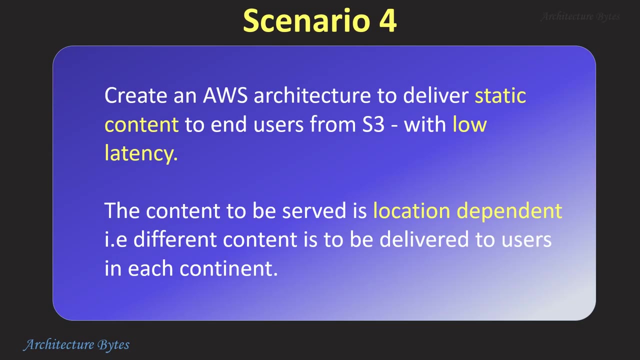 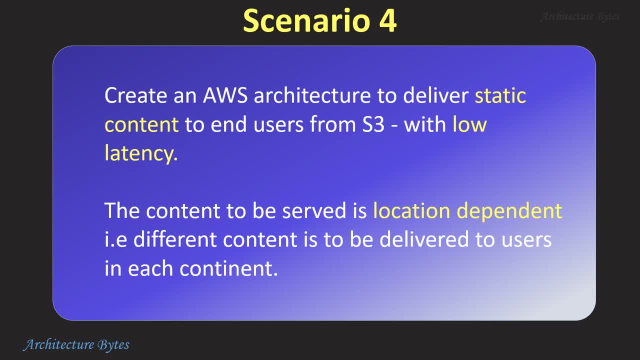 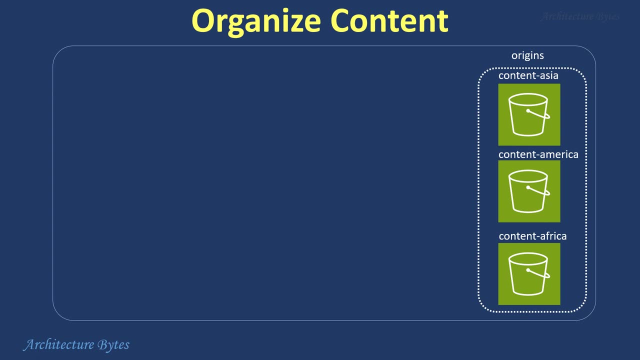 to end-users from S3 with low latency. The content to be served is location dependent. that is, different content is to be delivered to users in each continent. Organize the content in S3 geography wise, that is, in separate buckets or subfolders. This will serve as the origins for a CloudFront. 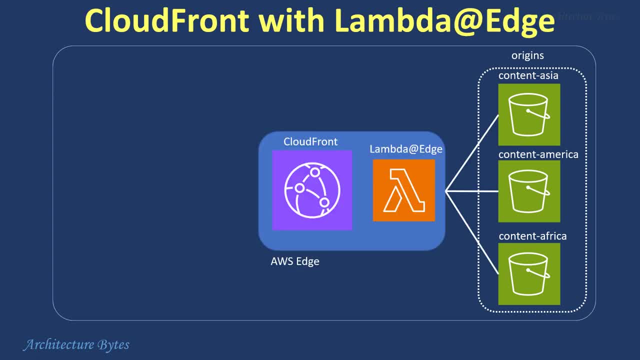 distribution. Next, create a CloudFront distribution with lambda at edge function that intercepts user requests and examines the HTTP header- CloudFront viewer country- to determine the user location and, based on that, switches the origin to be used. This ensures that correct application is available. 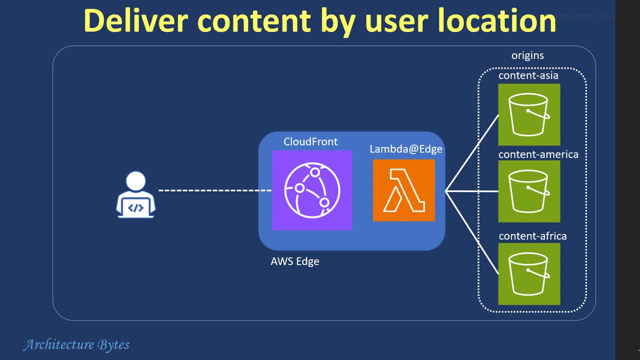 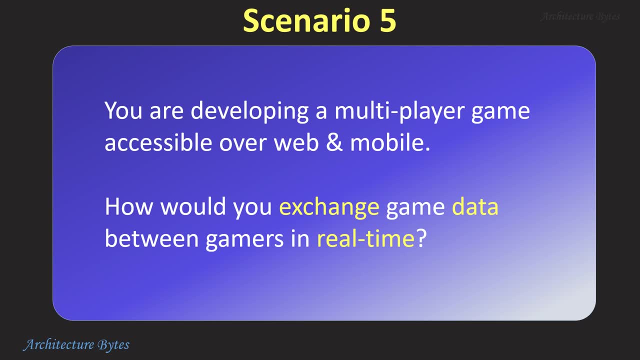 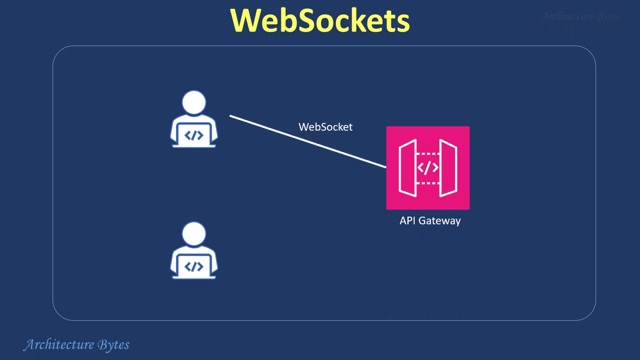 Location specific content is served via CloudFront. You are developing a multiplayer game accessible over web and mobile. How would you exchange game data between gamers in real time? You can use WebSockets to communicate with API Gateway. WebSockets is a communication protocol that enables a two-way real-time connection between a 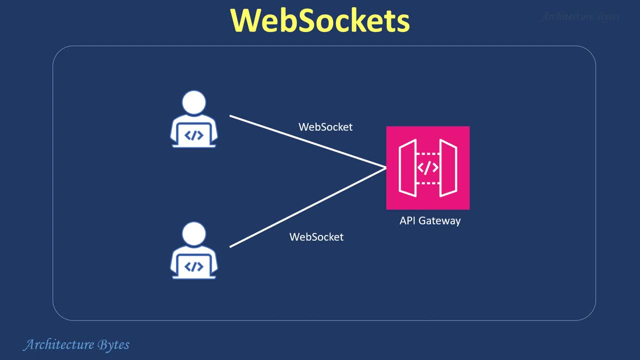 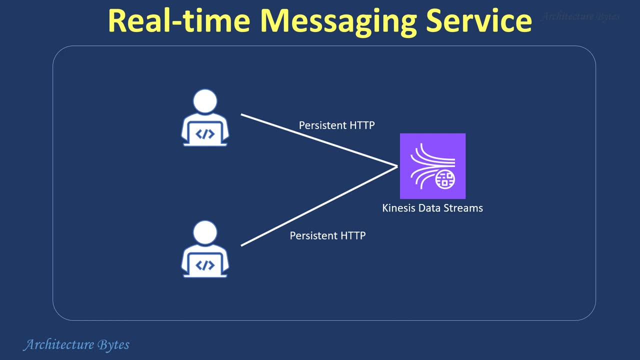 web browser or mobile app client and a server. You can use a service like Amazon Kinesis data streams, which acts as a message broker, allowing clients to publish updates and subscribe to receive updates from other players, or use AppSync to publish and receive messages over web. 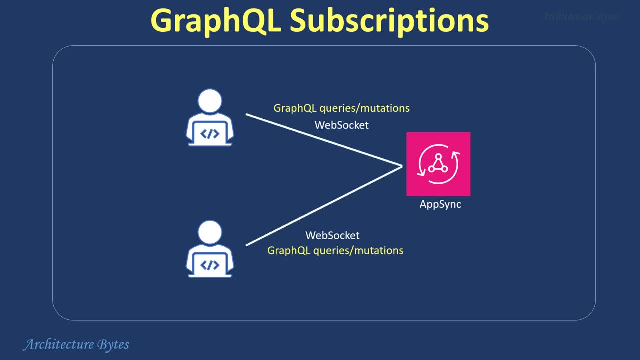 sockets. AppSync is a managed, serverless GraphQL API service from AWS. It allows you to define a GraphQL schema that represents your game data, like driver position actions, etc. Clients can use the GraphQL schema to define their game data. Clients can query and mutate the data using GraphQL queries and mutations. 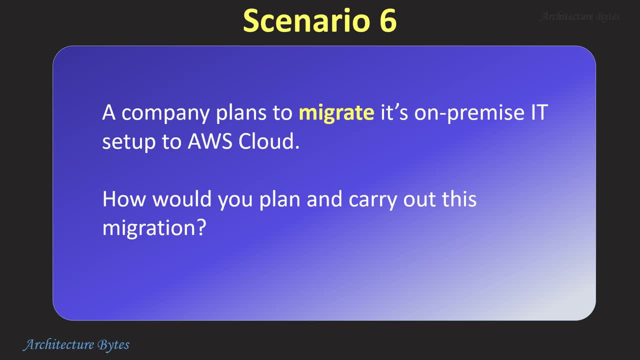 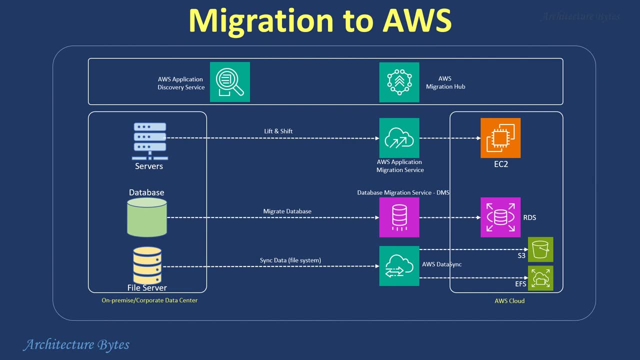 A company plans to migrate its on-premise IT setup to AWS cloud. How would you plan and carry out this migration? AWS provides several migration services to help us migrate workloads from on-premise data center or other cloud providers to AWS. Let's see how we can use them. The application discovery service helps. 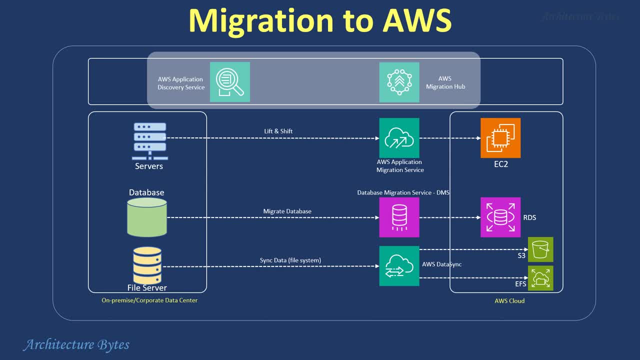 us collect information about servers and processes in the on-premise data center. The migration hub tracks and manages the overall migration process. For a lift-and-shift kind of migration of on-premise servers to EC2, AWS application migration service may be used. 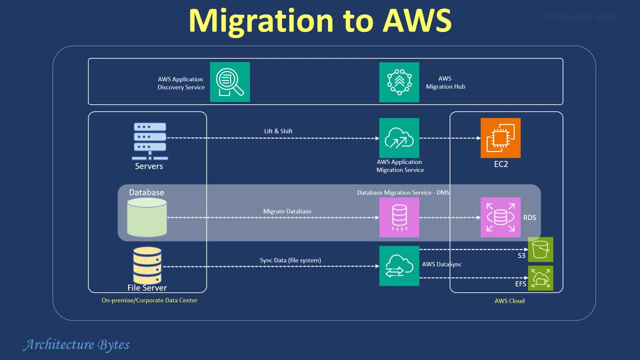 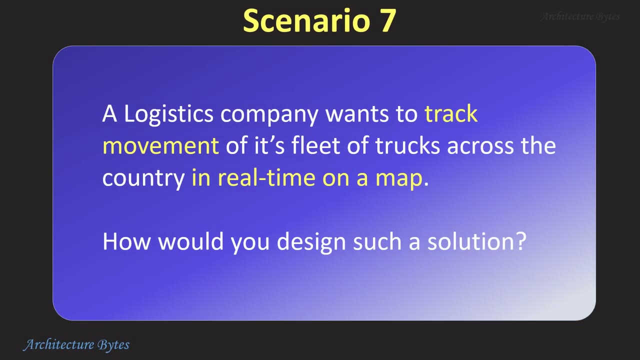 For database migration, DMS or database migration service is useful And for For file server copy and sync of data to AWS storage like S3 or EFS. AWS DataSync can be used. A logistics company wants to track movement of its fleet of trucks across the country in real time on a map. 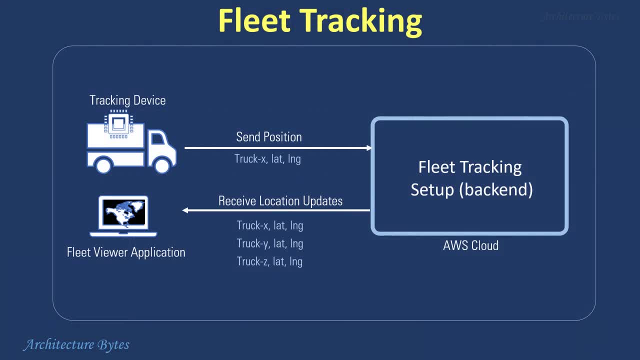 How would you design such a solution? Here's the overall flow. Every truck has a tracker device that sends its identity and geographical position every few seconds to our back-end tracking setup as a JSON message. The tracking device could be a dedicated IoT device or simply the mobile phone of the driver. 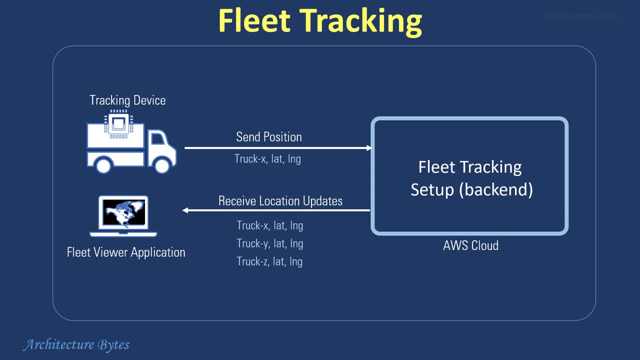 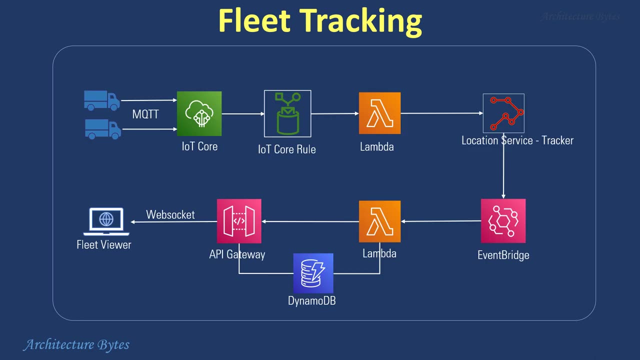 The fleet viewer application receives location updates for the trucks in real time from the back-end fleet tracking setup. The fleet viewer application will plot the location and movement of the entire truck fleet on a map. This is the same flow with service level details. Location updates from the trucks are sent over MQTT to AWS IoT Core message broker to a specific topic. 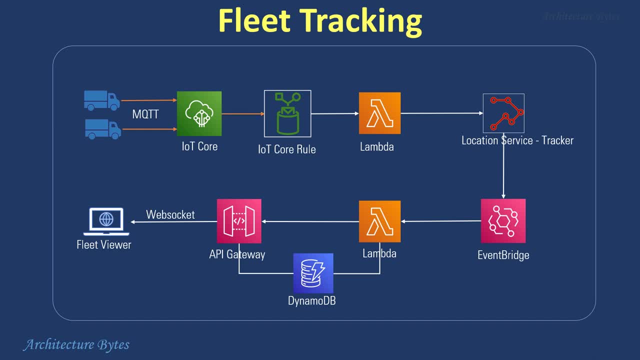 An IoT Core rule picks up the messages from the topic and invokes Lambda function which in turn sends the location updates to Amazon Location Service Tracker. The tracker saves the device location with itself and generates a geolocation update. event Event bridge captures the event And sends it to a Lambda function which sends messages to the fleet viewer application clients via the API gateway or WebSockets. 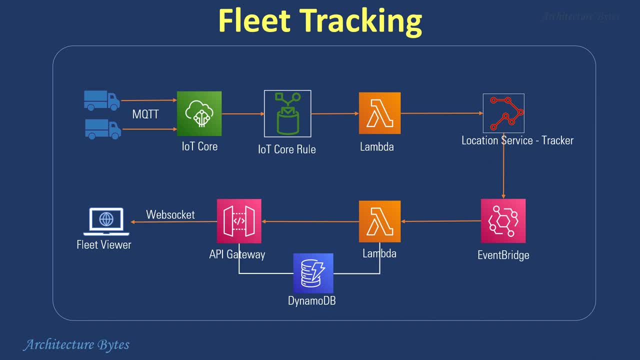 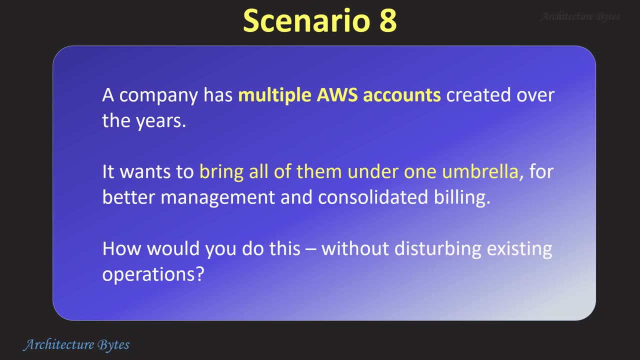 And thus the fleet viewer application receives and plots the truck fleet on a map. Note that the WebSocket connection IDs are saved in DynamoDB. A company has multiple AWS accounts created over the years. It wants to bring all of them under one umbrella for better management and consolidated billing. 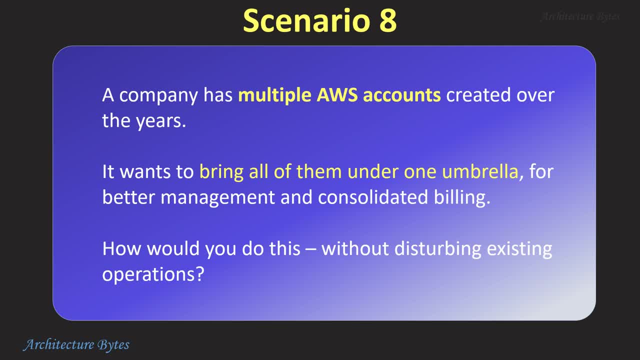 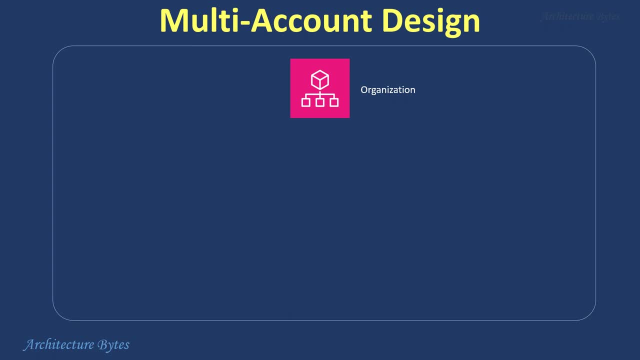 How would you do this Without disturbing existing operations? We will use AWS Organization Service to set up and manage multiple accounts. The primary account using which you create an organization becomes your management account, Under which you will create organization units or OUs, which are simply a convenient way to group accounts. 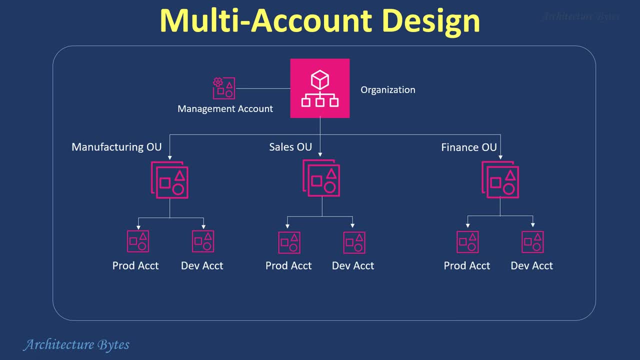 Under OU you can add other accounts- These can be new or existing accounts- which you would invite to join the Organization Service. These can be new or existing accounts which you would invite to join the Organization Service setup. once ready, you can do consolidated billing for all accounts at the